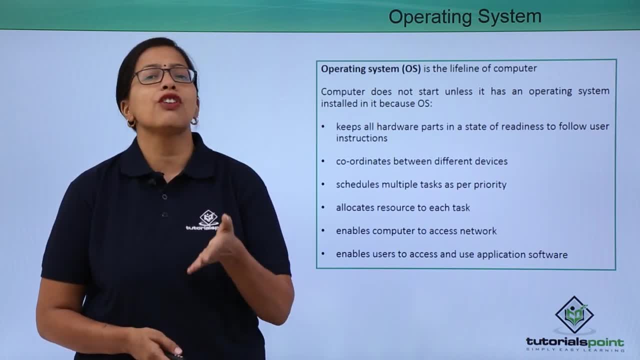 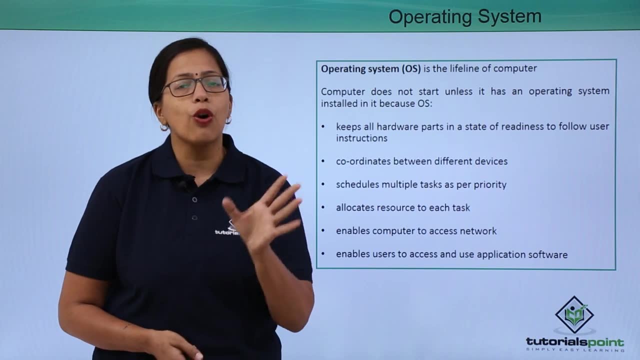 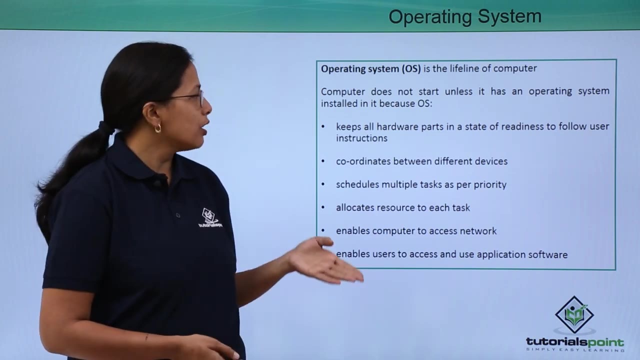 system is the lifeline of the computer because it cannot function without the operating system, As we have discussed in our previous video. also, operating system is always the first software that is loaded into the computer, Computer memory when it is switched of. why it is needed See keeps all hardware parts. 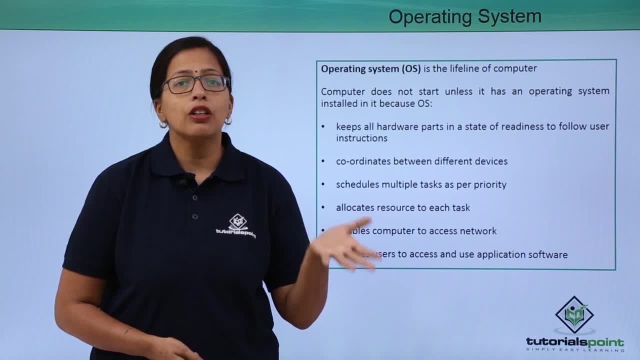 in state of readiness. So if I want to use a printer, the operating system will have the printer in a state of readiness. It is not that when I give a print instruction, after that the printer will be started and it will be ready to accept my instructions. It coordinates. 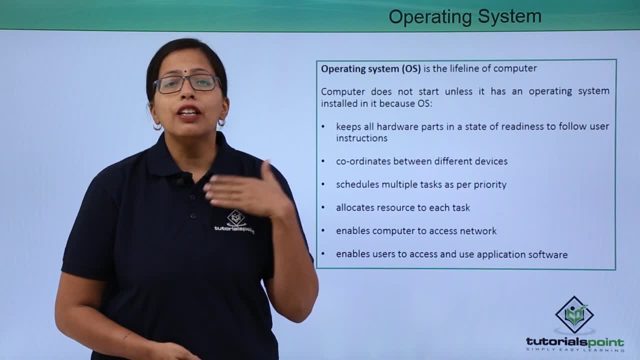 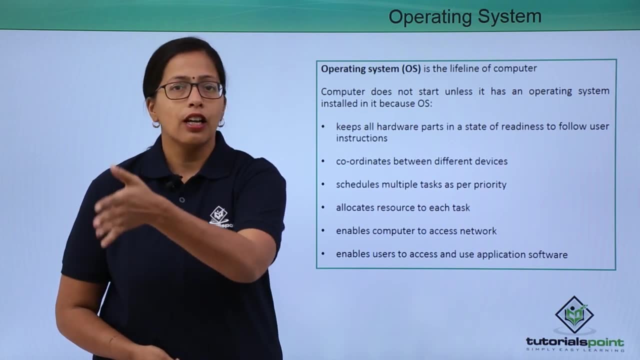 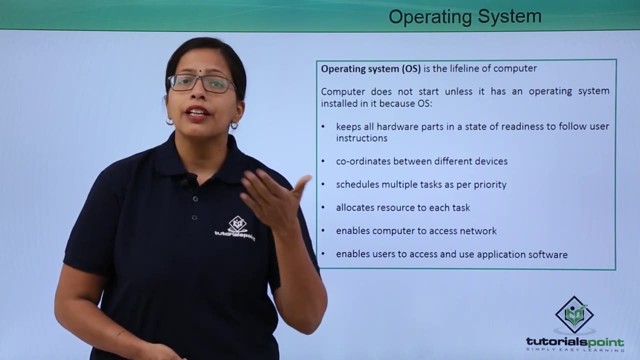 between different devices. I, as a user, will access only the control unit. The control unit, the operating system is, will coordinate with other devices, other output devices or the memory units, and vice versa, when those units need to interact with me: give me an output, give me an error message. 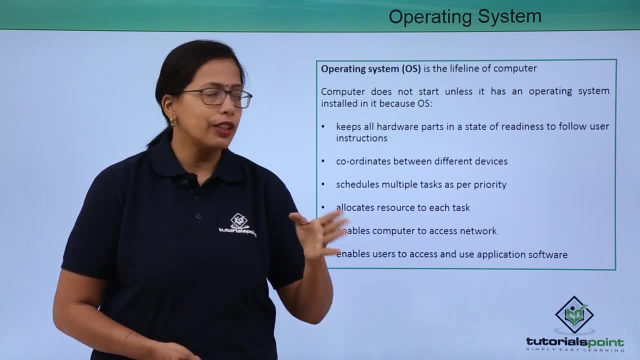 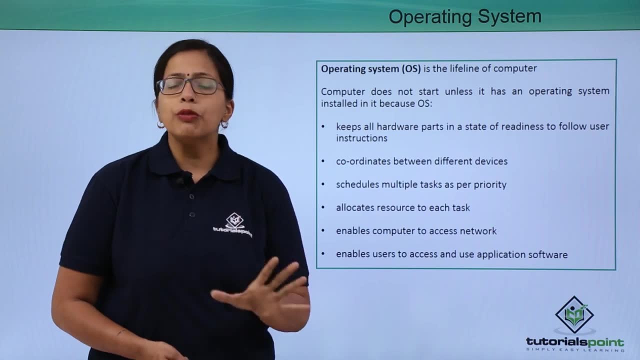 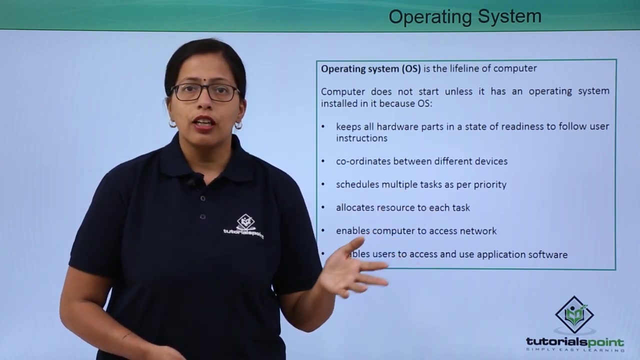 they will do so through the control unit or the operating system. it schedules multiple tasks as per priority. now, at any given point of time, computer is doing multiple tasks. let me give a small example which you might have been doing yourself. suppose you are reading your project report on the system. simultaneously you have opened your email box and then suddenly you see: 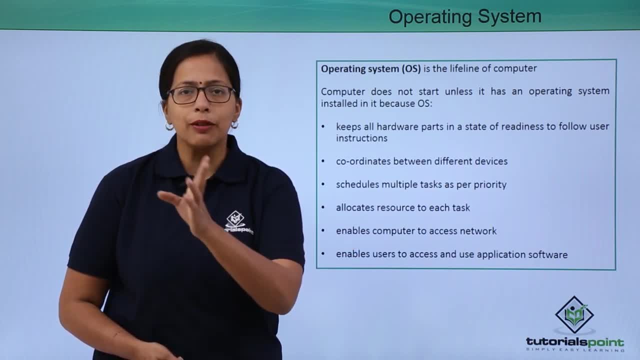 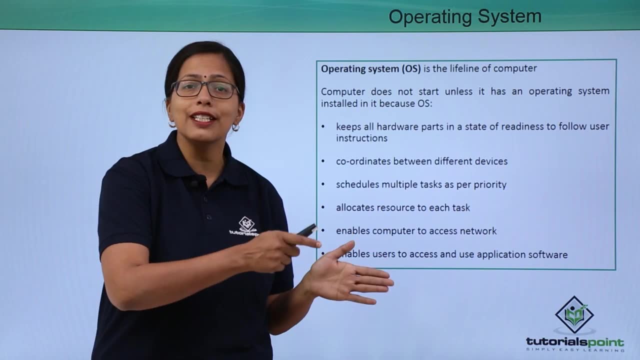 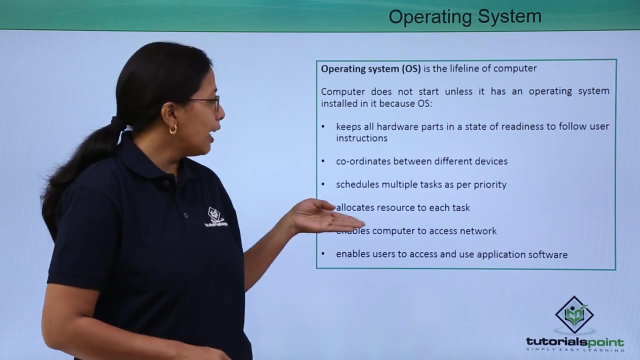 your chat messenger popping up. so you might be doing them one by one, because when you are reading your project report you will not be chatting, but the computer has to handle all these simultaneously. it's the operating system that decides the scheduling of all these tasks it allocates. 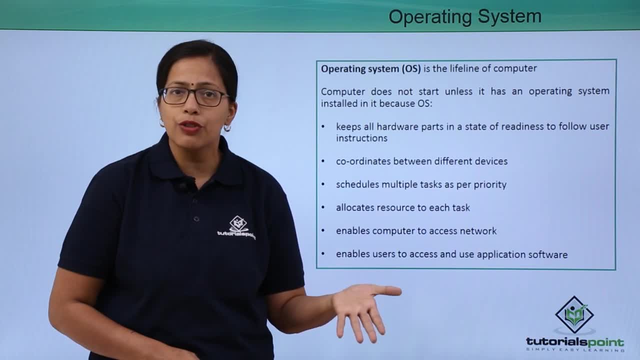 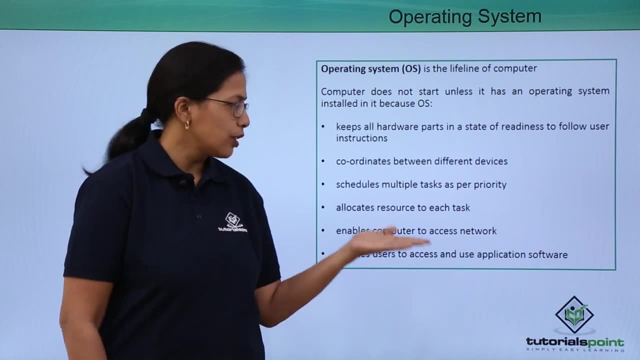 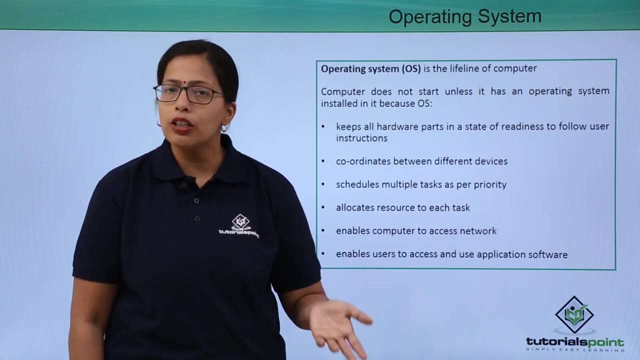 resources to each task. each task would need some resources: some window space, some disk space, some printer space. OS is what decides all this. it enables the computer to access the network. when you want to attach your computer to the internet or a local network, then OS is what that does it. 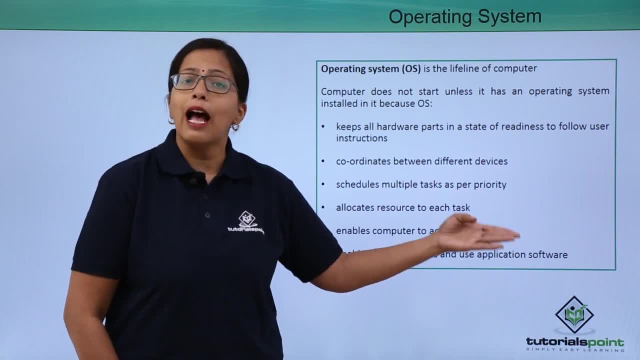 it enables user to access and use the application. software OS is the interface. these are some of the important things that you need to know about the operating system, so let's move on to the next one. these are some of the important things that you need to know about the operating system, so let's go to the next one.